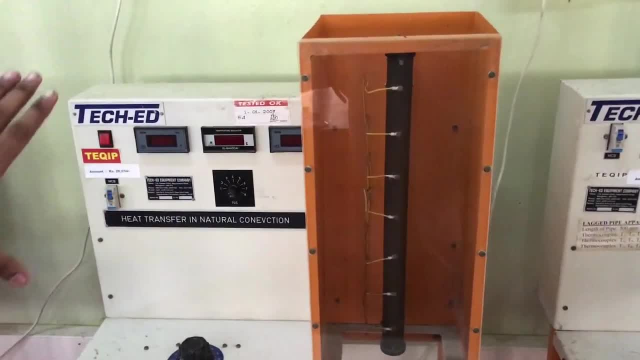 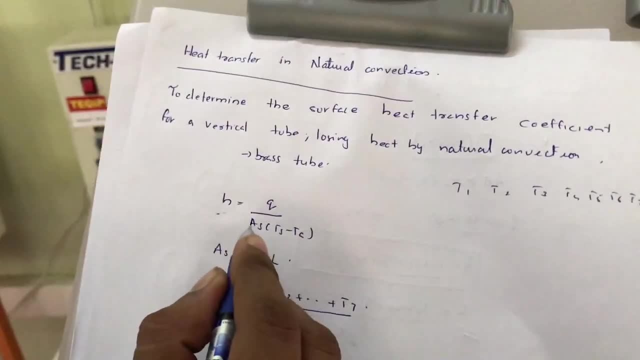 are having the surface temperature of that brass tube and if you are having the ambient temperature, then look, this heat transfer coefficient is equal to Q by area of surface area As into Ts minus Ta. So here we are having the surface temperature of that brass tube and if you are having the 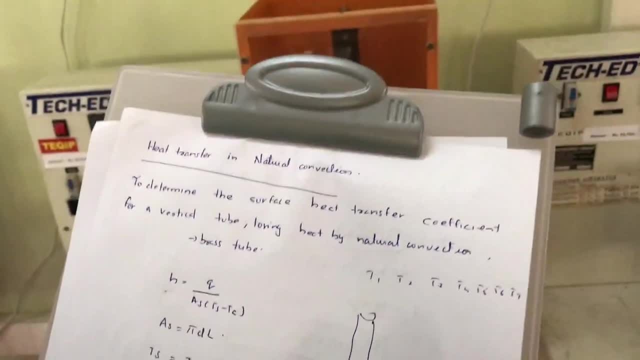 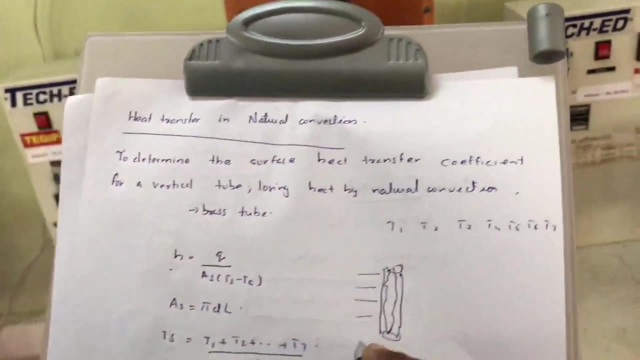 ambient temperature of that brass tube and if you are having the ambient temperature of that brass tube and if you are having the ambient temperature of that brass tube, and here we are having a brass tube and inside this brass tube a heating coil is kept and seven thermocouples are kept on the surface of this brass tube and we are supplying heat. 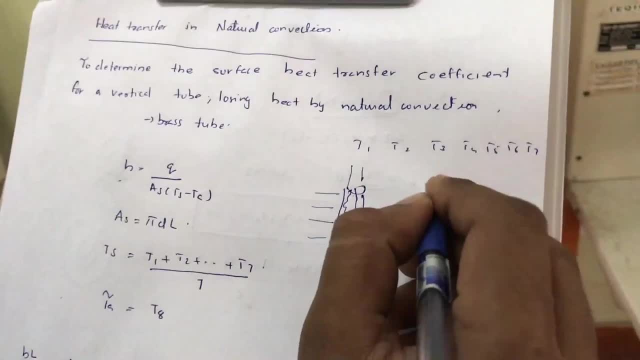 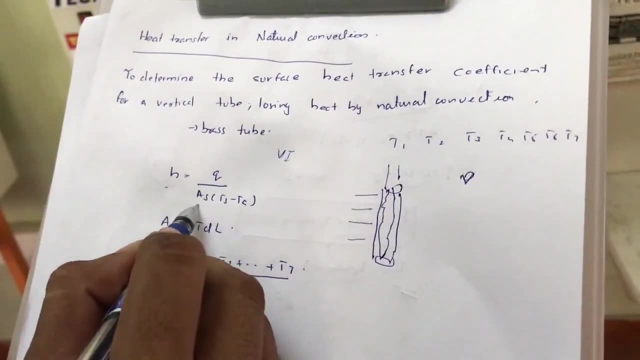 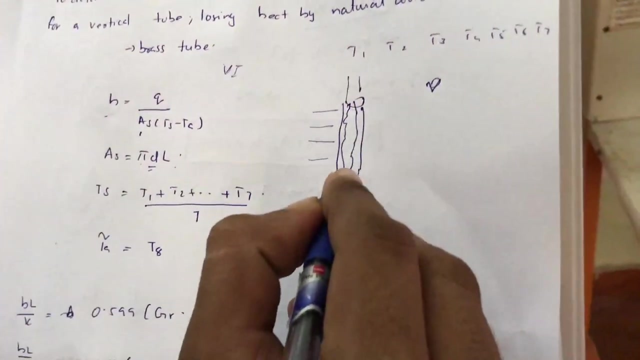 energy to this coil and if you are having knowing the voltage and current, we can find Q. Q is equal to V. into I, Then surface area of the coil As surface area of the brass tube, that is, Phi into D1.. into n, where d is the diameter of this brass tube and l is the length of this brass tube, which are 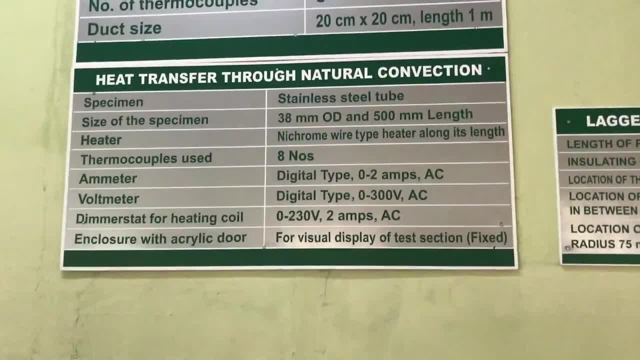 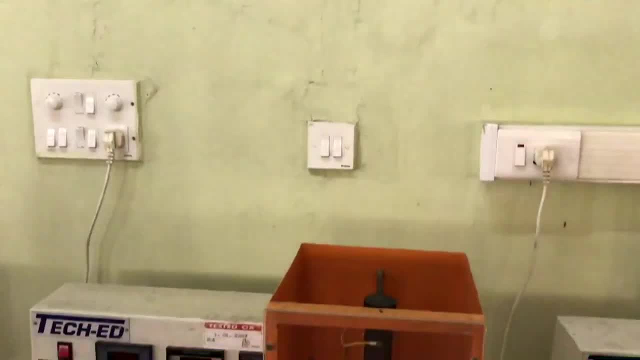 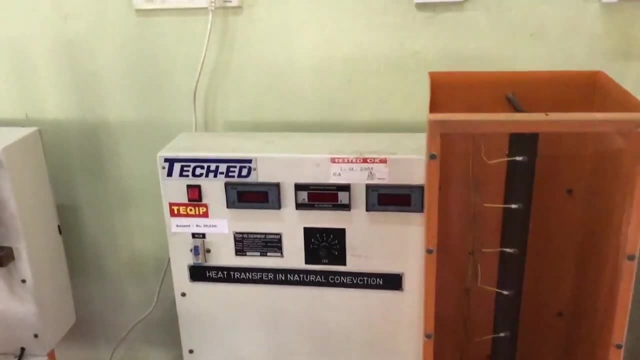 which can be obtained from the specification of this brass tube. so diameter is 38 mm and length is 500 mm. so now q is v into i. so if we are able to obtain that v, i and temperature, we can find heat transfer coefficient. so first we will be sitting on this main switch and then mcb. 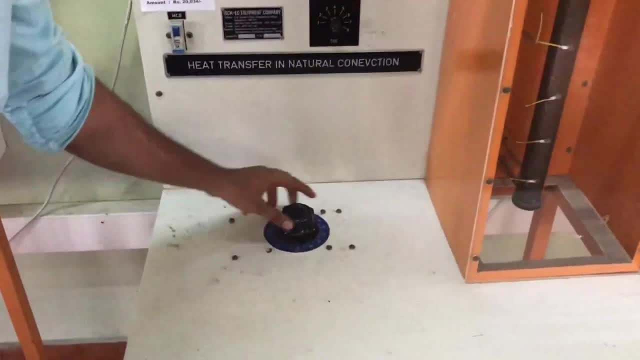 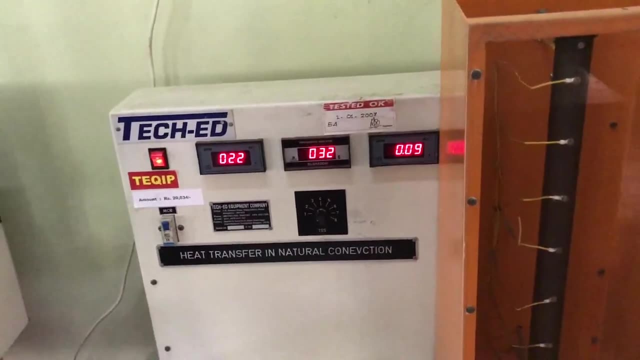 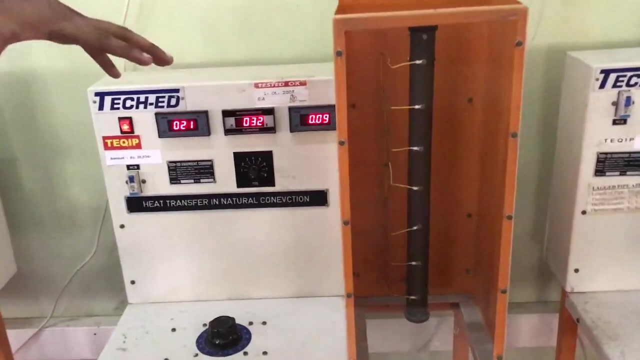 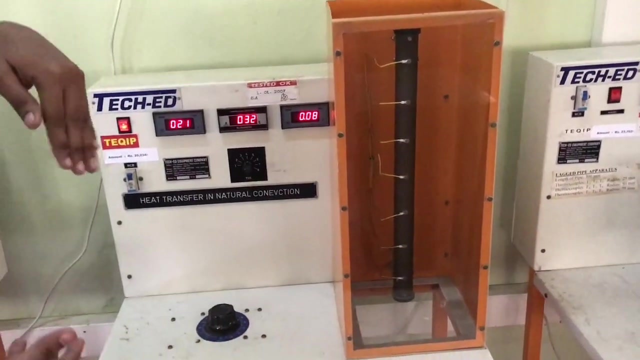 then the panel switch. okay, initially this dimmer stat should be at zero, should be at zero. and then what we do is: uh, inside this coil. this coil is having about a uh, it's having a capacity to hold about 100 watt, so we are mainly the heat supplied inside that 100 watt by adjusting the voltage. 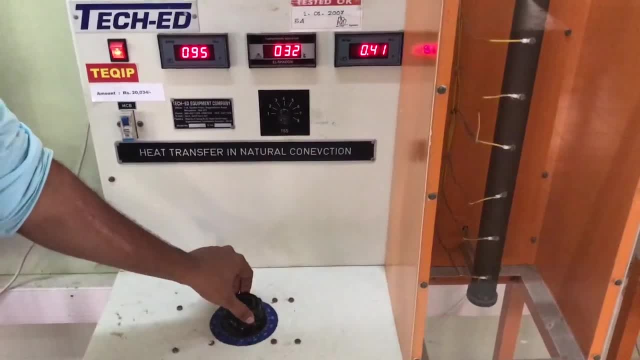 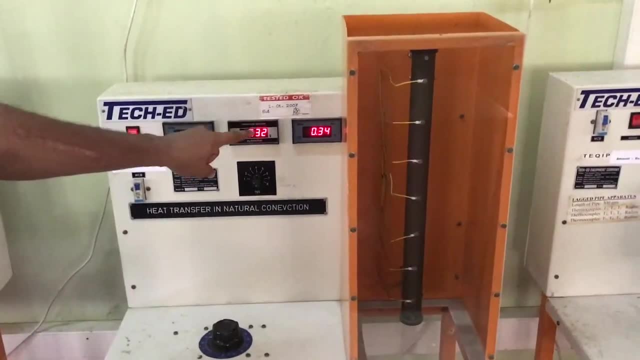 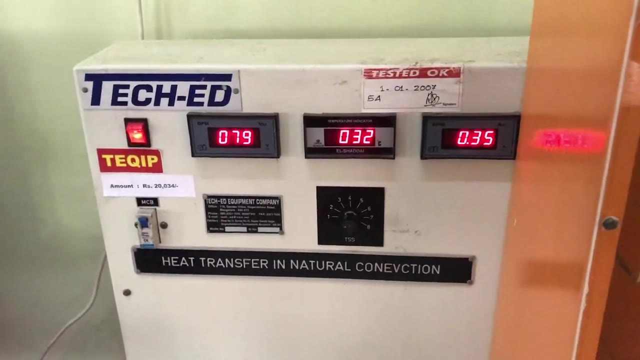 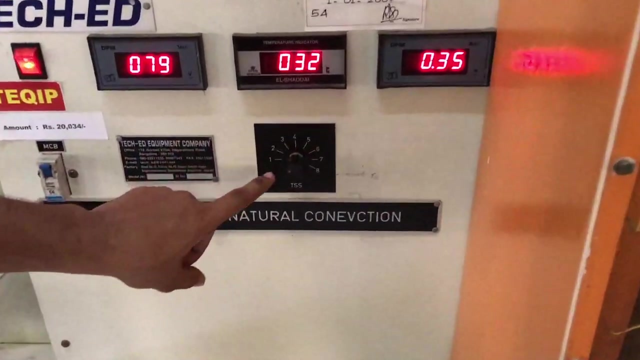 so let's keep that voltage at, say, 80 watt. so okay, it's 79, 79, and the current is about 0.35. that means the power supplied is about 24 ohm. that's okay, it's, it's under safe condition. so now here we are having the readings of thermocouple this: knob shows the reading of termocouple. is the read temperature. so if we look at source temperature, here is the temperature of thermocouple. this knob shows the temperature of thermocouple. here is the temperature of thermocouple. so if we x, then it is set to zero. so it is set to zero. 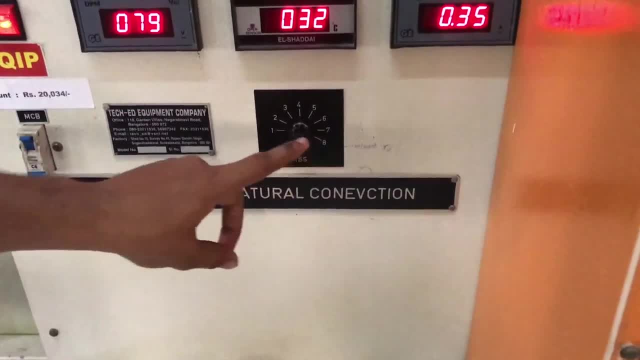 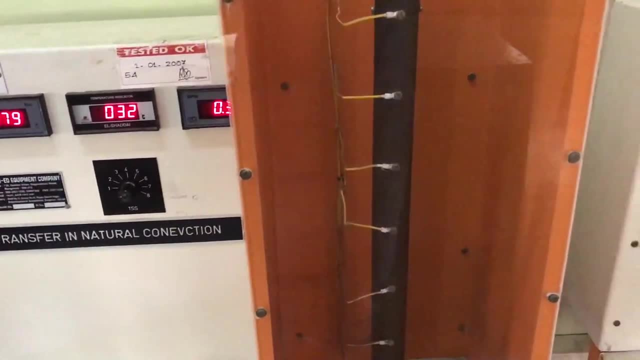 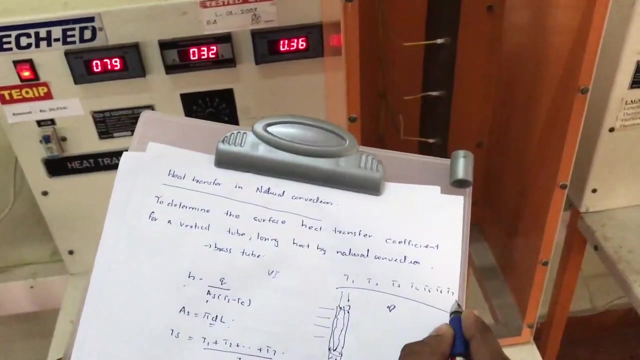 the thermocouples: 8 thermocouple, of which 1 to 7 represent the thermocouples on the surface of the brass tube, and the 8 thermocouple represent the ambient condition. So what we do is we are having a column like this: T1 to T7 and then T8, T8 is the ambient. 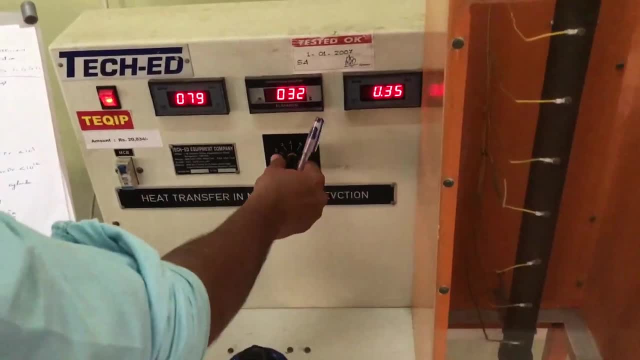 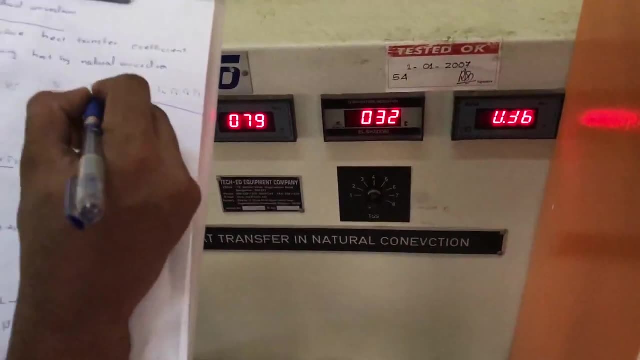 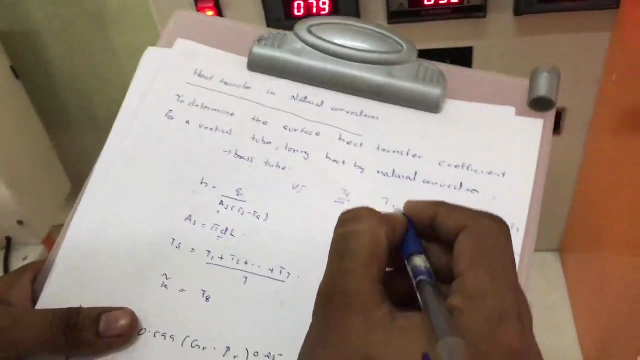 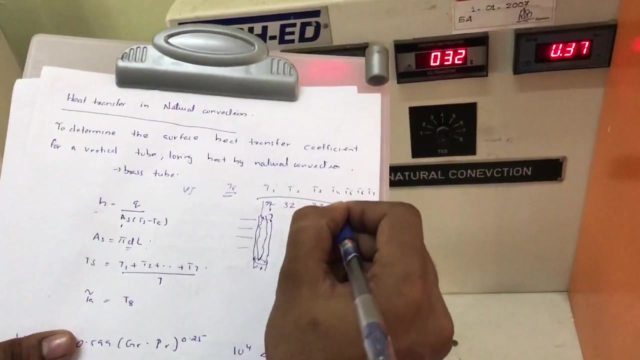 condition. that will be same. So we will be taking the reading: initially T1,, so T1 is 32 degree, then T2, T3, like that we will be taking the reading. So now we have T1, 32, T2, 32, T3, 32, now T4, again 32, T5, like that we will be taking the. 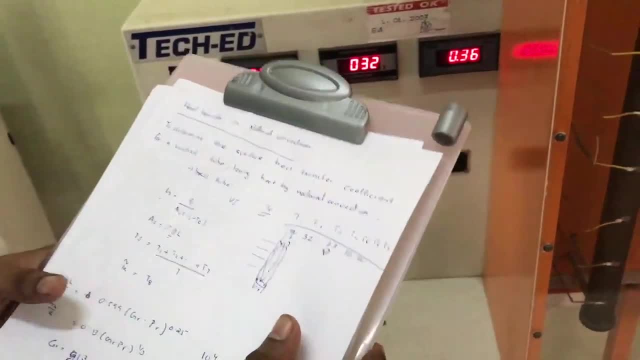 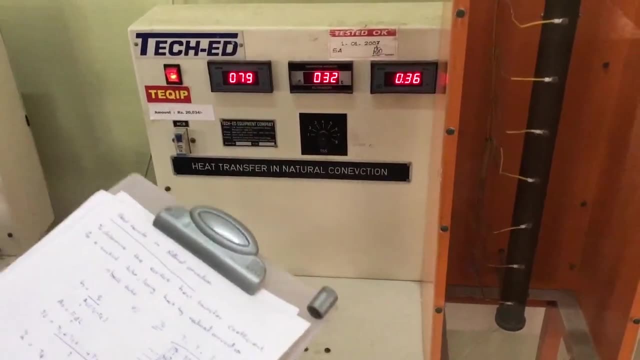 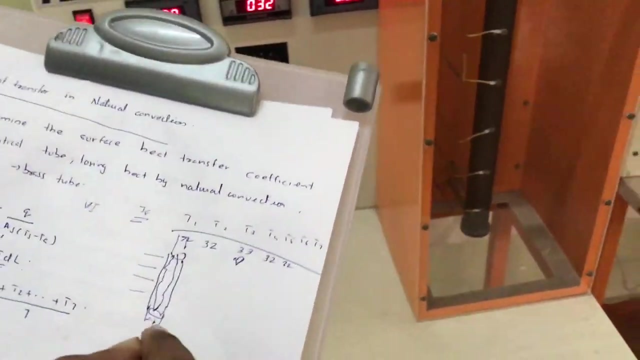 reading. So after taking the first set of reading, we will be taking the next set after 10 minutes. So we will be taking readings after the interval of 10 minutes and at last a state will come when the suppose say: now the reading is 31,, 32, like that, 33, etc. and at last a state. 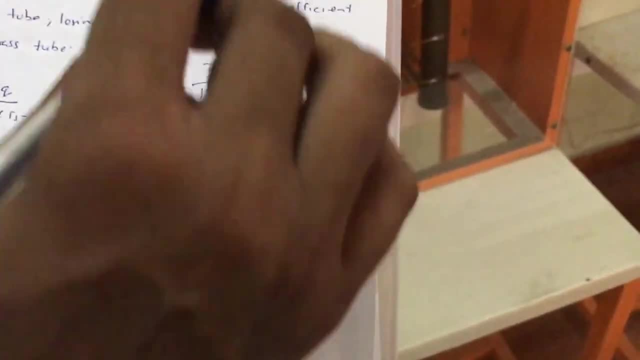 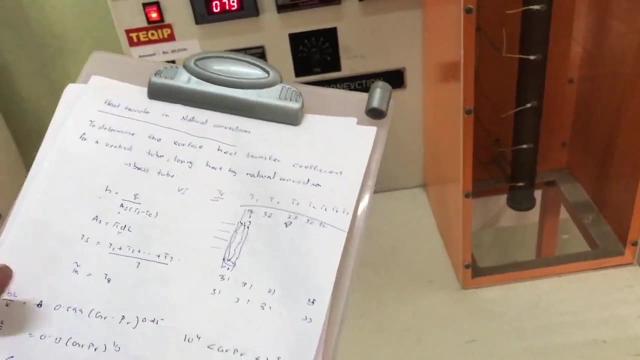 will come when the readings of that particular set will be same as that of the previous set. That means now it have reached a steady state condition And at that time we can take the. So we will be taking the average of first 7 thermocouples, that is, T1 to T7, and we can 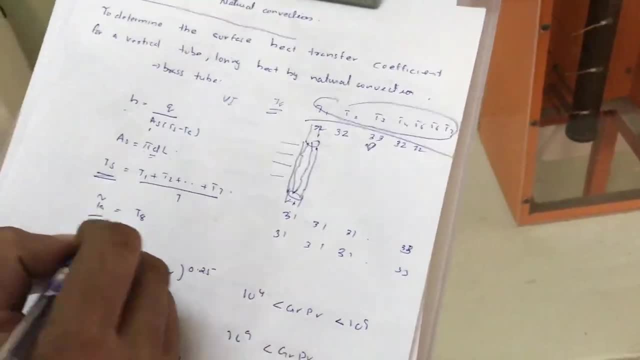 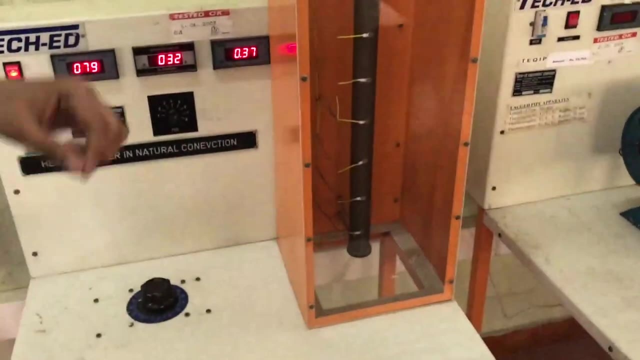 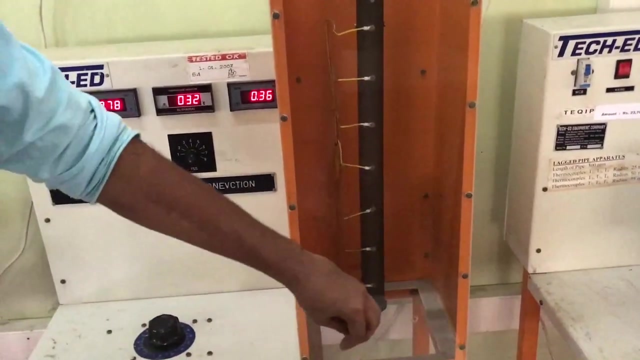 find, the surface temperature And ambient temperature will be obtained by the reading of the 8th thermocouple. And then so here, what happens is, from inside the coil, heat will be emanating to the surface by convection, and so what happens is, because of this heat, density of the air will be decreasing. 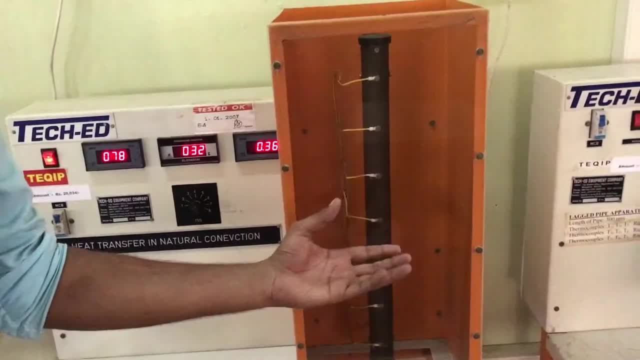 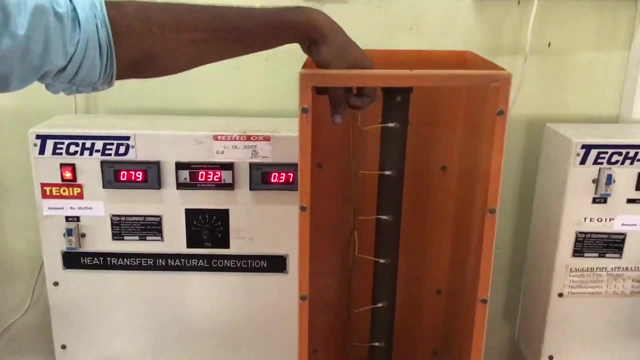 So air will rise up And because of rising of air, So the temperature will be decreasing, More air will be pushed towards the lower side, from the lower side, and because of that this air will be carrying heat outside and the natural convection occurs. 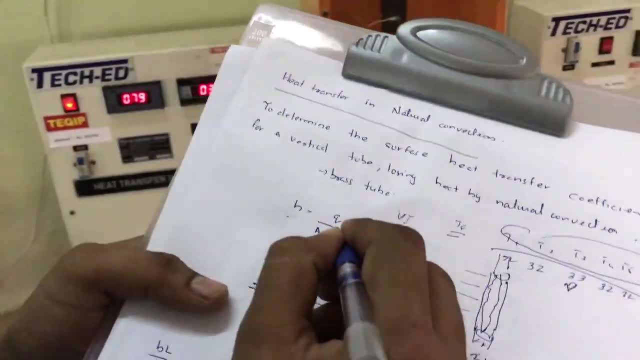 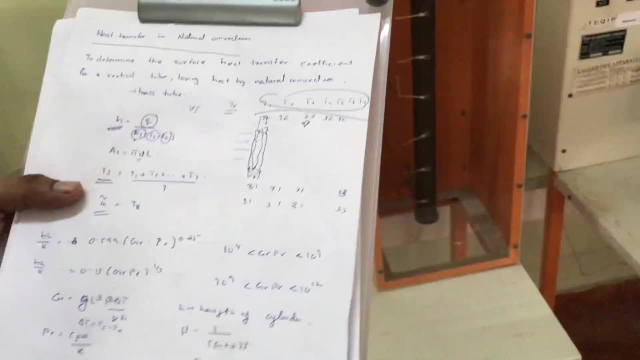 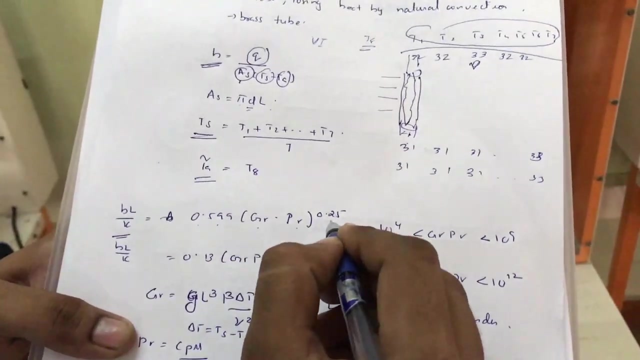 That's what happens here. So we are able to obtain Ts, Ta, and Q is V into I, As is pi, dL. So now we are able to obtain the heat transfer coefficient, And now HL by K is equal to 0.59, into pressure of number, into planetary number, into 0.25..